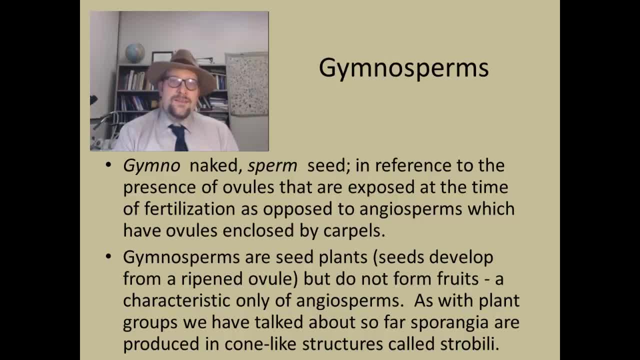 root gym or gymneo, which means naked. This is the same root that we get gymnastics and gymnasium, and the reason for that is that the Greeks used to perform sporting events naked. Now Spurm is in reference to seeds in plants, Now the reason they are called. 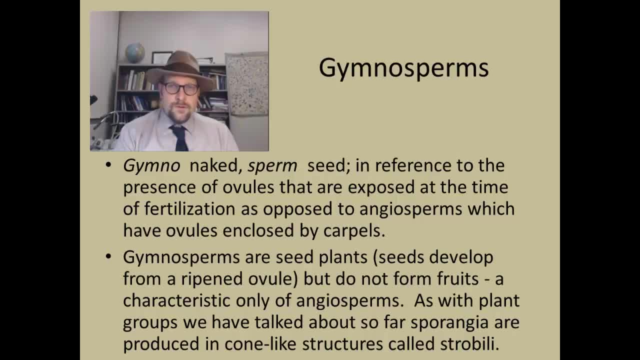 naked seed plants is because the ovules are exposed at the time of fertilization rather than being enclosed by carpals. Now, ovules are the smallest section within the plant receptor. the plant gets fertilized by pollen, which ripens the pigments. Theiezera vorstellens one of the 12 ovules perceived to be naked. 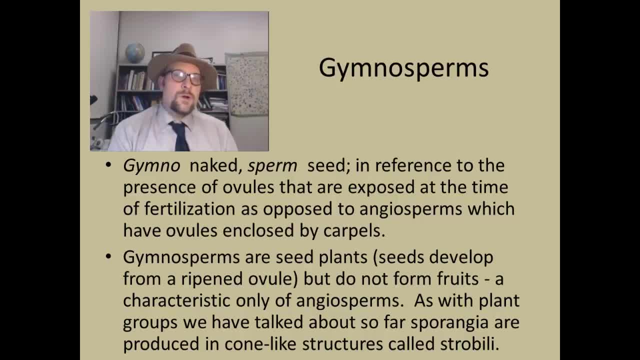 and the egg is shown to be the only remaining part in the egg cluster. These ovules are into the seeds. Germiosperms do not form fruits, and we will talk about the sporangia that are produced and restricted to cone-like structures called the strombula or strombulus in the singular. 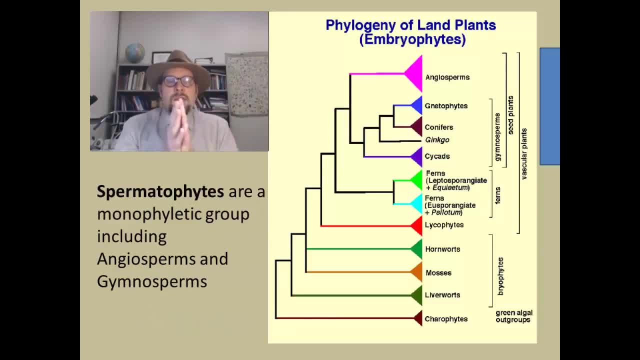 We can group these more advanced seed plants into a single monophyletic group of plants which include the cycads, ginkgos, conifers, juniophytes and angiosperms. Hence, the germiosperms are a polyphyletic group, likely ancestral to the angiosperms. 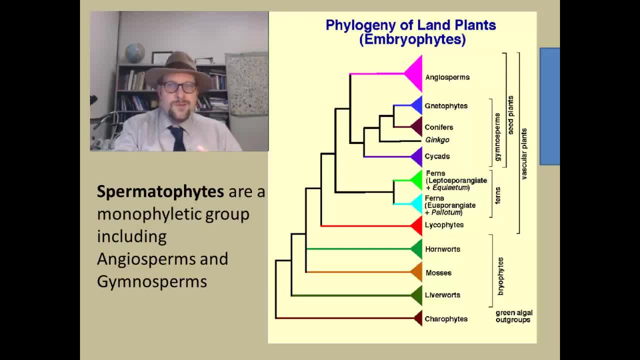 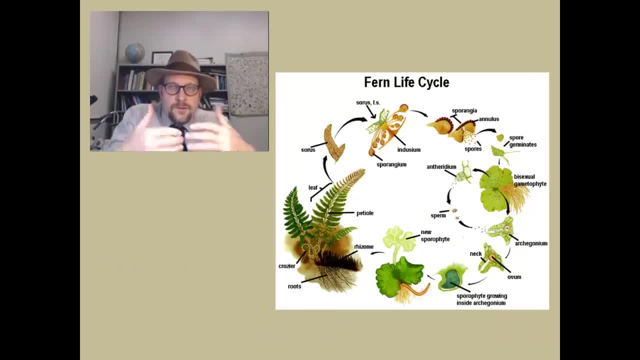 Germiosperms include many of the evergreen trees such as conifers and junipers, but they also include a few deciduous trees like ginkgos. The origin of seed plants from spore-bearing plants was a really big innovation in the evolution of plants. 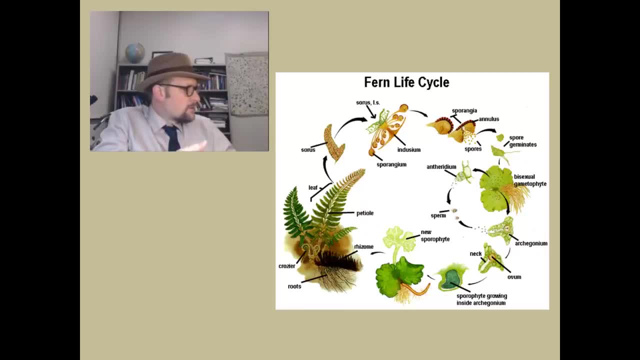 Here we have the typical life cycle of a fern. Remember that ferns produce spores, and these spores fall to the ground and grow into this gamiphyte generation. These are tiny little plants that sole function is in the sexual reproduction of the plant. 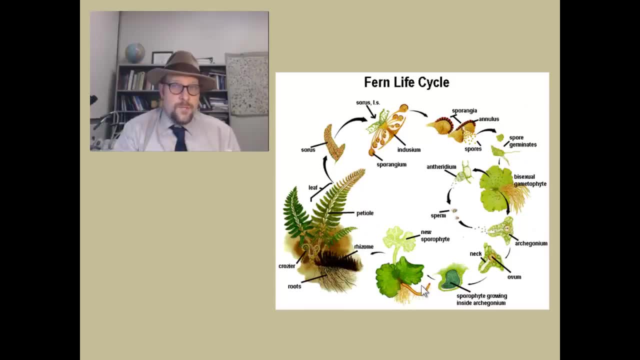 The gamiphyte contains both male and female parts, with the male parts being the antherium and producing the flagellated sperm. They swim in the water to reach the archegodium, which contains the eggs. Once fertilized, these eggs grow into a zygote and eventually into a new fern plant. 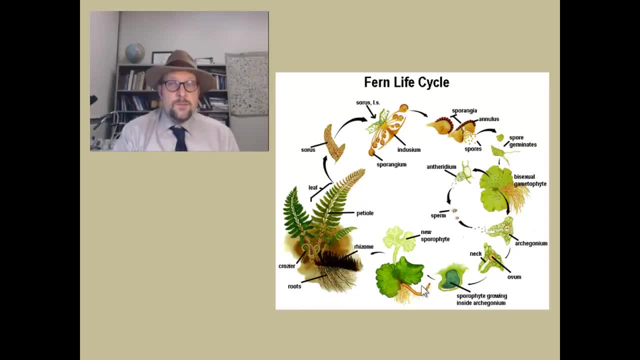 Sexual reproduction occurs in the water, and hence ferns have a limited habitat for wet environments, or at least seasonally wet environments. The evolution of a mechanism to forgo this whole requirement of sexual reproduction in the water would be a major advantage. This would allow plants to become fully independent of these wet climates. 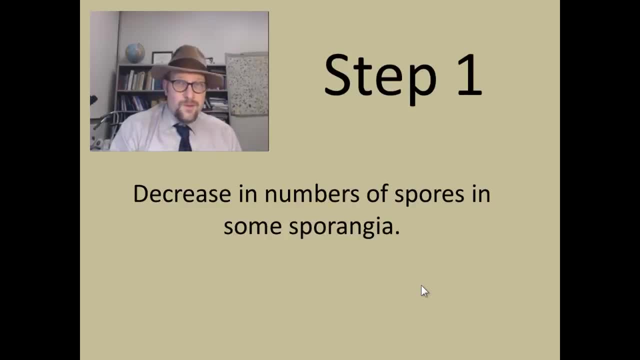 Let's go through the steps towards developing seeds that we would have to go through The first step, step 1, is a decrease in the number of spores in some of the sporengia. These are followed by step 2,, which is an increase in the size of the remaining spores. 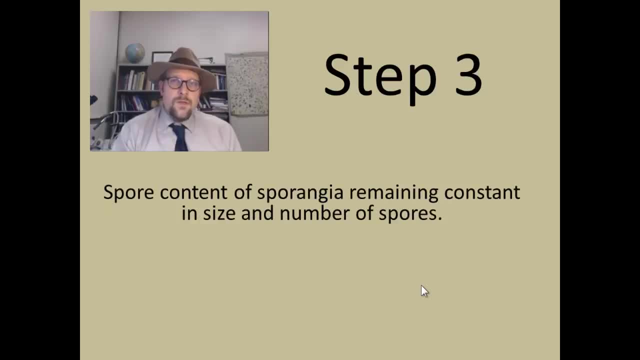 Plants would have bigger and fewer spores. The third step would be that these spores would have a consistent number. They would be of a larger size on the plant. The fourth step would involve the change from monocerous gamophytes. those are gamophytes. 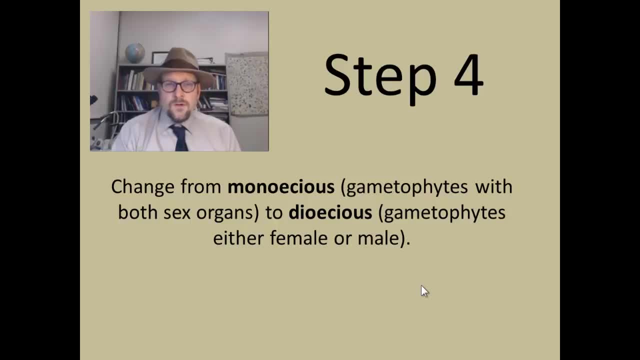 with both sex organs, and that's what you see in a lot of ferns to a dicerous. those are gamophytes that have either male or female parts. We've seen this in some of the bryophytes, where the gamophytes were in separate sexes. 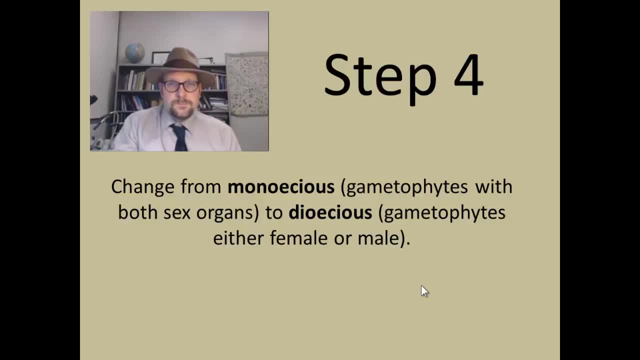 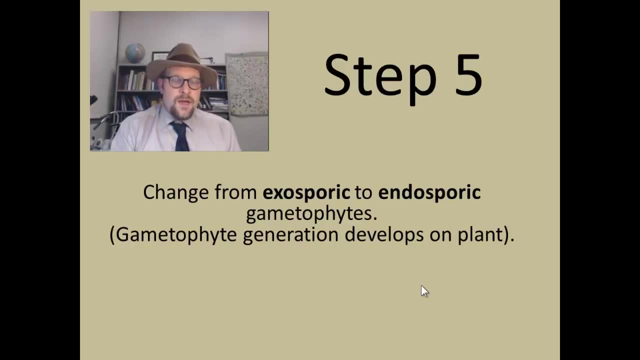 but this is going to be in some of these bigger plants. Next step- this is the biggest step- when the gamophytes develop on the plant rather than being shed off the plant, This means that the gamophyte generation is retrained on the sporophyte generation. so 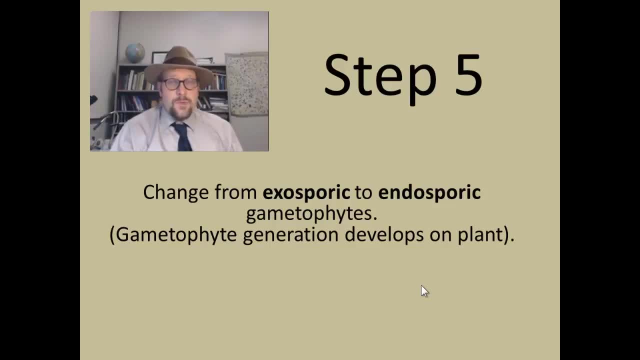 this is a major reversal of roles between the two generation of a plant's life cycle. thus the gamophyte becomes to important part of the above-ground plant. Nun What Where? We will look for this transition in the fossil record and attempt to see how seeds originated. 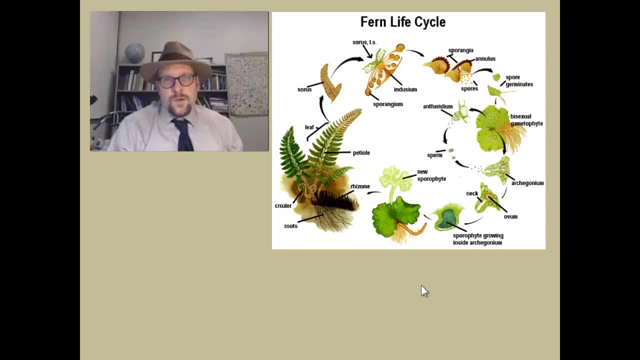 in plants following these steps. This is a major switch from the fern life cycle, that is, the retention of the gamophytes, these parts of the life cycle, on the actual plant itself, on the sporophyte generation. These gamophytes are going to look and act very differently than what we see in ferns. 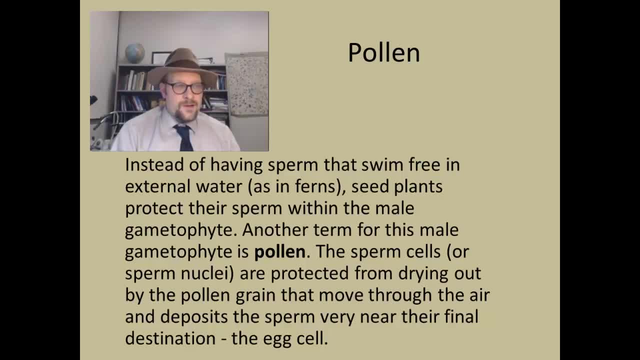 What, then, is pollen? if it is not a spore, is it the sperm? Instead of having phylogenated sperm that require water to swim, seed plants protect the sperm within the male gamophyte, so a male gamophyte is pollen, the entire thing. 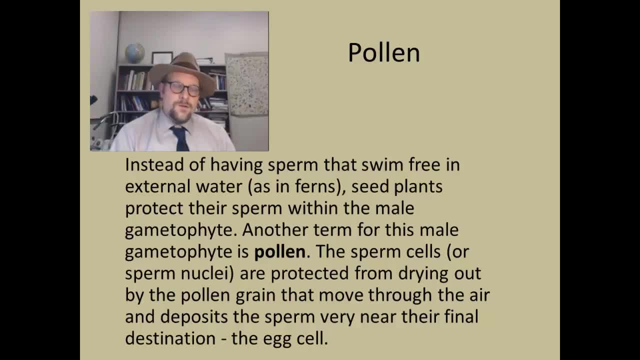 is pollen. That is really weird. The sperm cells or sperm nuclei are protected by other cells within the pollen, which help move the pollen through the air so that it can be deposited into the ovia and the female gamophyte generation, which contains the egg cell. 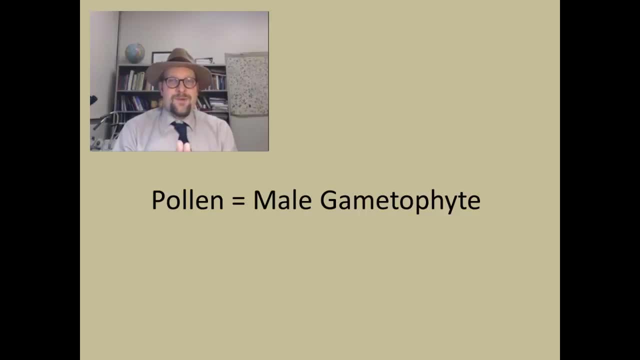 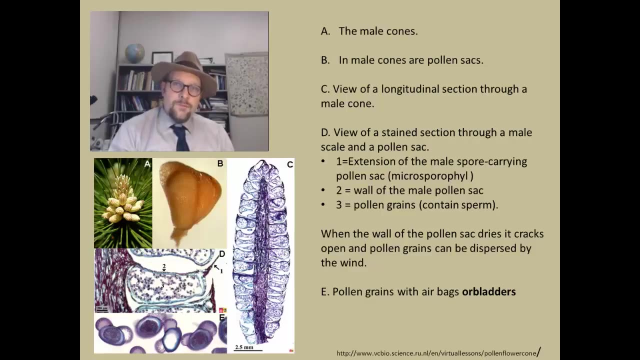 To reinforce this idea, pollen is the male gamophyte. that is pretty cool. Let's look at some of these structures on a modern conifer. We have male and female. The male cones produce the sporangia that hold onto the spores which actually develop. 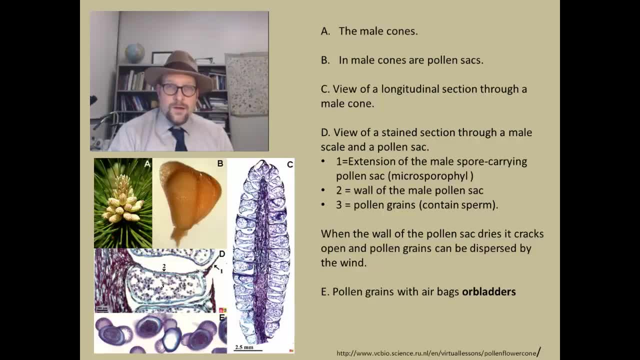 into pollen sacs that contain thousands of tiny pollen. This is a cross section of a typical cone showing each of these pollen sacs that are inside. When the plant dries in the height of summer, they will split open and burst and release. 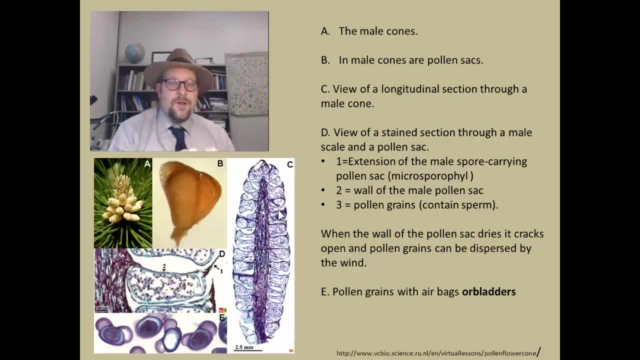 these millions and trillions of pollen- These pollens are the gamophyte generation- being sent out into the air. Here are some pictures of the pollen down here and they kind of look like little Mickey Mouse ears, because they have little ears on either side. 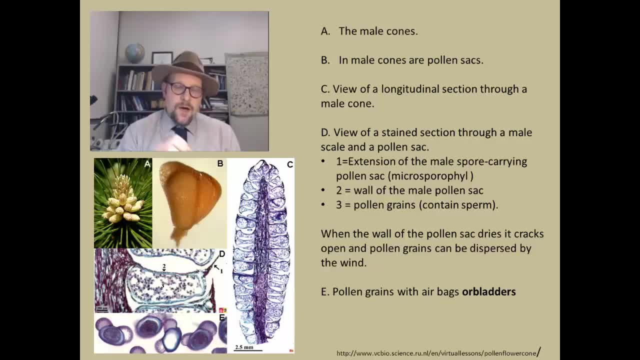 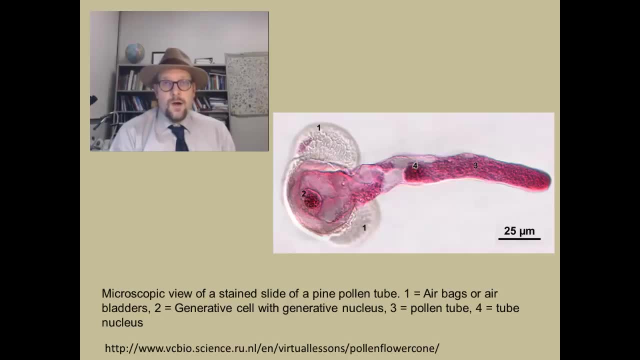 These are actually airbags or aura bladders and they actually help the pollen be dispersed in the air. Here is a microscopic view of a pine pollen, and note that, in addition to these little Mickey Mouse ears that you see, with a lot of conifer pollen in particular, you also 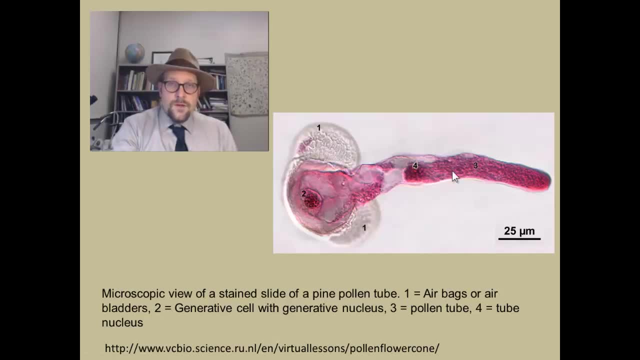 see this tube that comes out here, this long tube. That long tube is called the pollen tube and this tube is going to be important when the pollen comes and actually fertilizes the egg that's in the ovula, in the female cones of the plants. 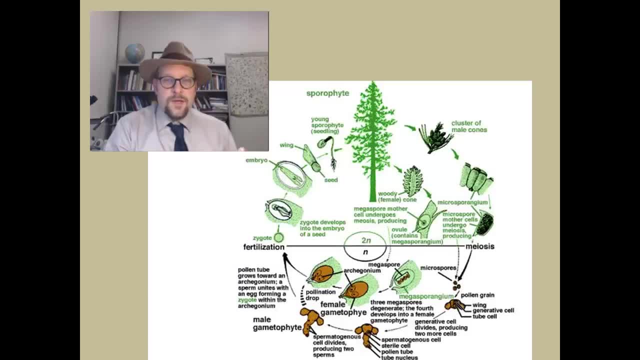 Now let's take a look at the life cycle of a typical gymnosperm like a pine tree. It is very different. The male and female cones on the plant retain the gamophyte generation, and the female cones contain what are called the megasporangia. so these are spores that are going to be very 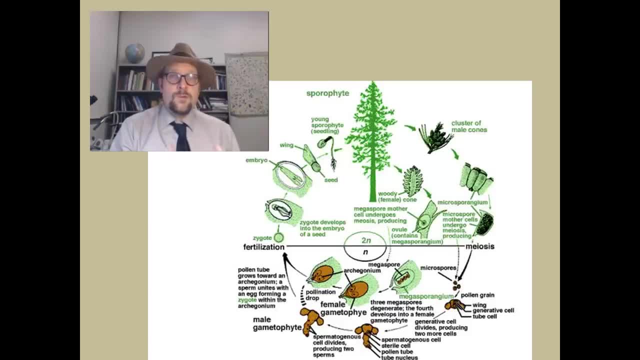 big. Those spores are going to grow into the female gamophytes with an archegodium that contains an egg cell. The male cones contain what are called the microsporangia. This is the egg cell. This is the female. 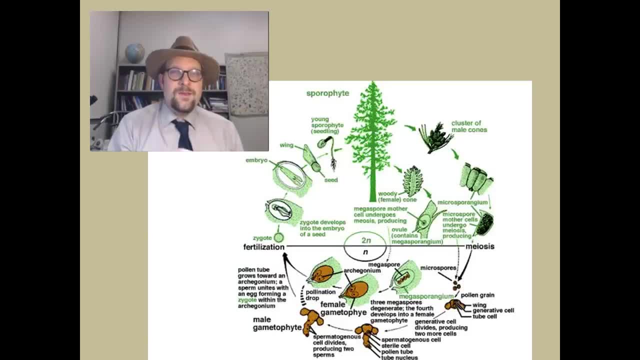 This is the spores. This is the spores. These spores are going to grow into the male gamophytes. Those male gamophytes are the same thing as pollen. The pollen is released in massive quantities into the air. they float around and then 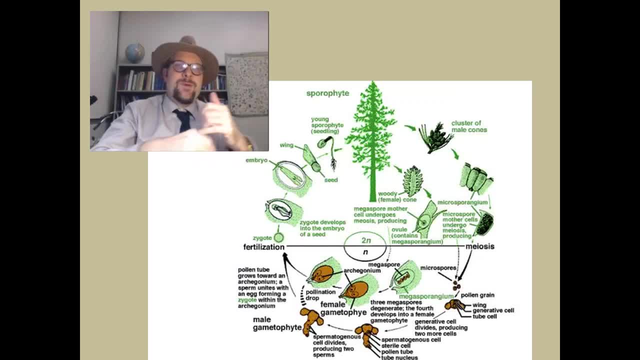 they happen to fall onto the female cone. The female cone is then fertilized to form a zygote encased in a seed. Then the seed is shed and that seed can grow into a new plant. This is what we see with a lot of these seed plants. 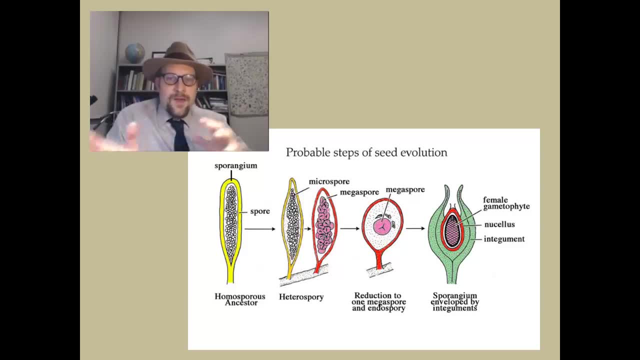 Now let's look at the hypothesized evolution of seed plants. In the first stage, we have a sporengium that is referred to as homospores, Homo spores, Homo spores, Homospores, Homo spores, Homo spores. 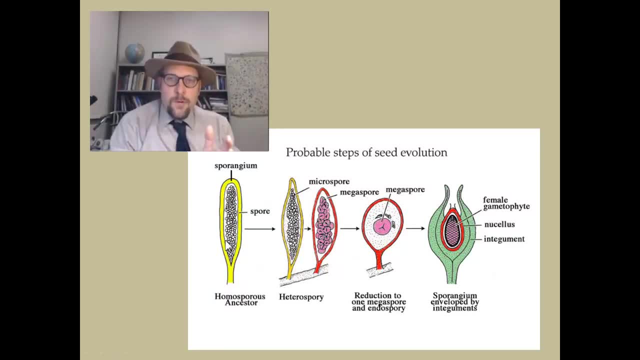 All the spores in the sporengium look the same, even though some of them would develop into female or male plants, or into plants that have both female and male parts on them. Then we have to move to the next stage. The next stage is the stage where we have two different types of spores on the plant. 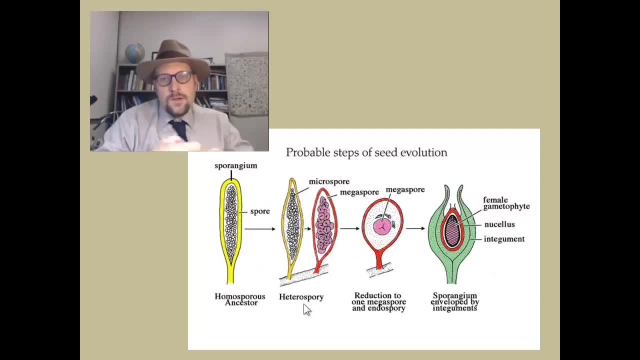 Spores, that are microspores and megaspores. spores and the microspores are the ones that develop into the pollen eventually. And then we go to the next step here, where that megaspore gets reduced and it retains. 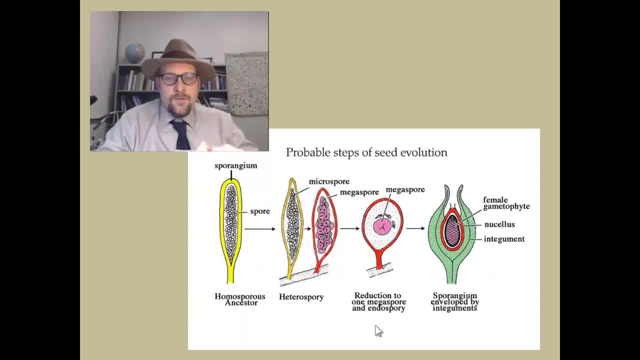 itself on the plant so that it grows into a gamophyte, and this means that the egg is encased in the archegodium of the gamophyte that is held onto the plant, and we refer to that as endospore. 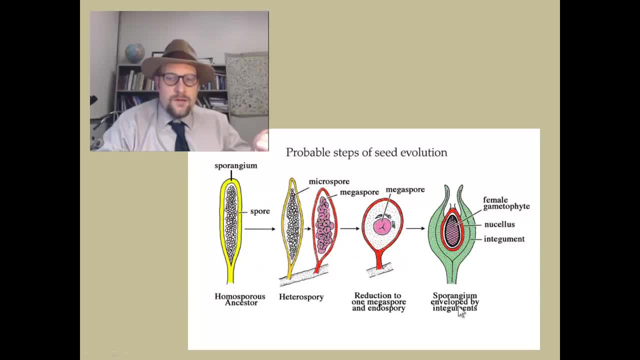 And then, eventually, we get this very important stage where we get the megaspore gets encased by a cup-like structure that is called the ovium, and that is where the female gamophyte resides, and that cup-like shape is what is going to catch the pollen that is blown out. 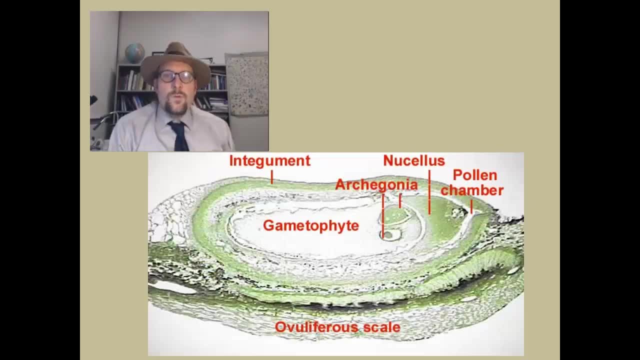 to the wind. Here is a thin section through one of these female gamophytes and here we see a greatly reduced archegodium within the ovula and it has an egg cell and we see a pollen chamber right here and this is where the pollen will come down and grow and then invaginate into. 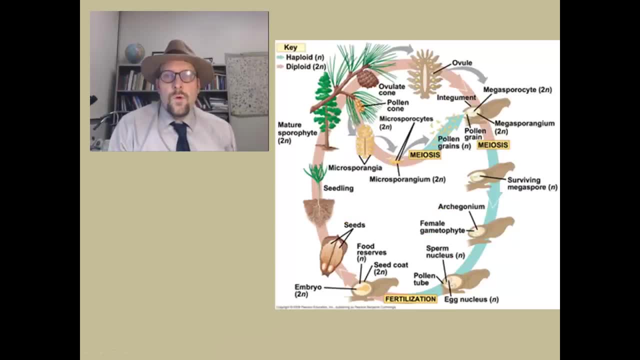 the nucleus of the egg for fertilization. The other thing to remember is that once this egg cell in the female gamophyte is fertilized, it will form into a seed rather than a plant. Seeds are a pretty novel innovation and, as we will see, will have a profound effect on 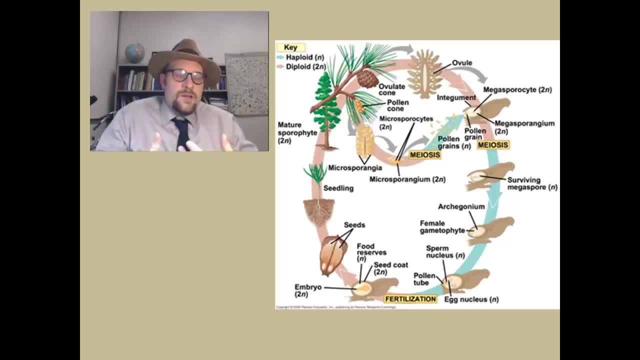 the flora and fauna of the world and this is a major innovation to really get away from wet climates and a wet environment. By doing this, these plants are really becoming fully terrestrial and start to take over some of these drier climates And get rid of these dry climates. 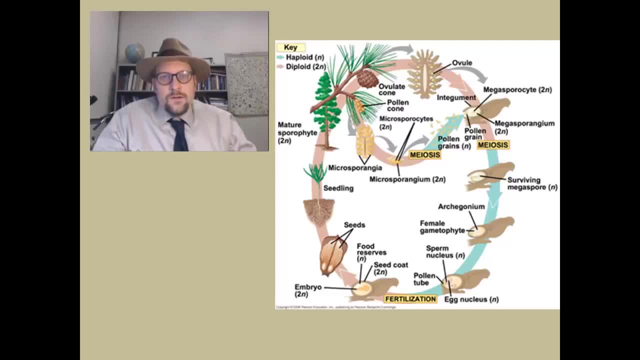 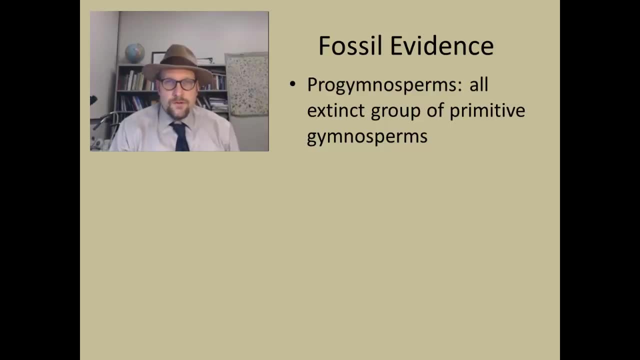 And get rid of these dry climates. Get rid of these dry climates Now. many of these transitions are preserved in the fossil record in a group of fossil plants called protogymenia sperms. These plants are the ancestors of modern gymnaia sperms and show the acquisition of many traits. 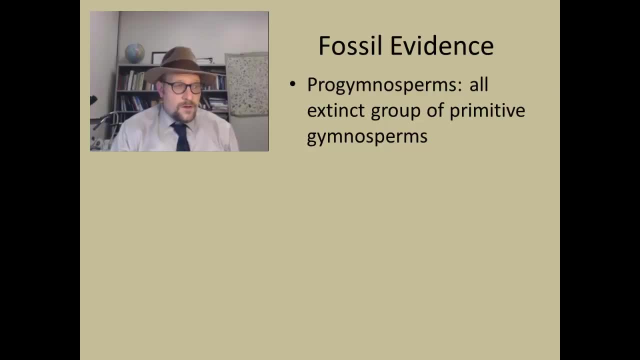 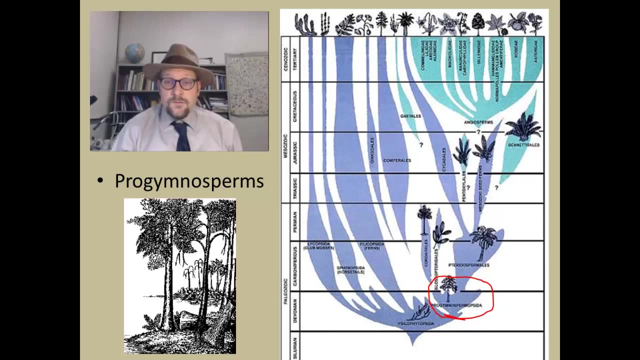 Protogymenia sperms are all extinct, but their fossil record extends all the way back to the Devonian Protogymenia sperms. Protogymenia sperms here split off very early in the evolution of plants and throughout the Carboniferous. 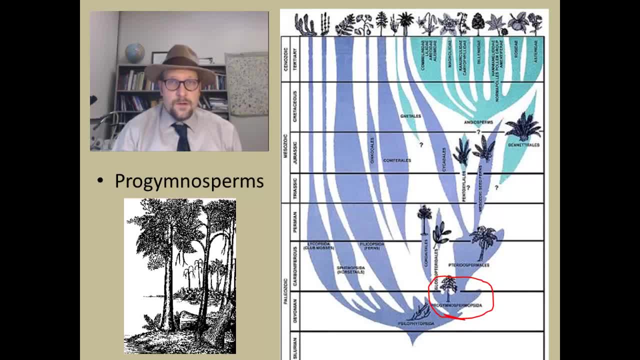 they also split into various groups of plants we will talk about. By the end of the Carboniferous, the major groups of gymnosperms split and will all go on to become very successful. these include the conifers, the cycads, the ginkgos and 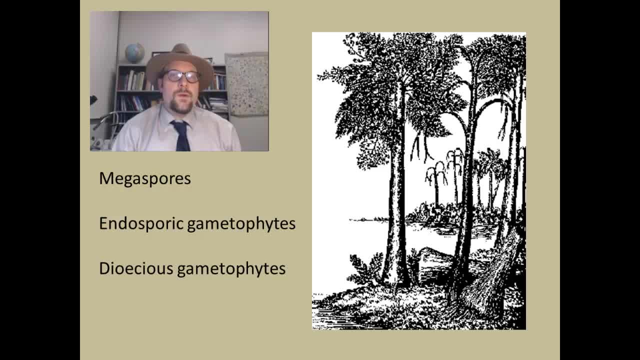 some unusual groups we will discuss later. We want to look for some evidence among these proto-gymnosperms, of things we have mentioned before. We will look for Megaspores, so spores that are much bigger than we have seen before. We will see for endosporic gamophytes. these are going to be where the gamophytes are retained. 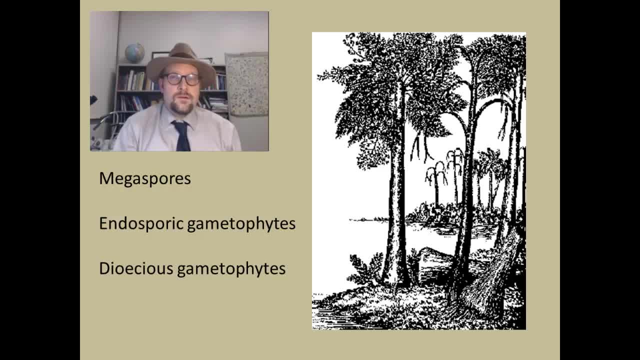 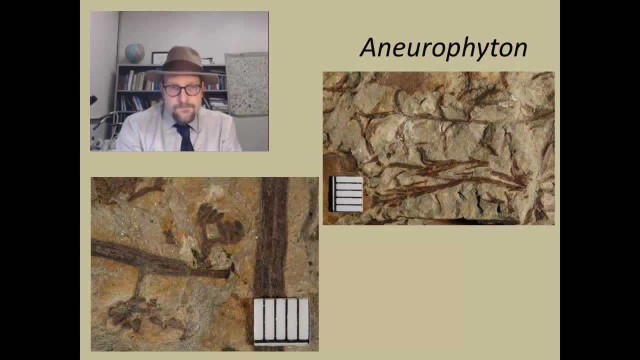 on the plant. We are also going to look for disigeous gamophytes. Alright, so here we are. we are going to cross our fingers and here is hoping that there is some really complete fossils. Here is the first fossil plant we are going to look at. 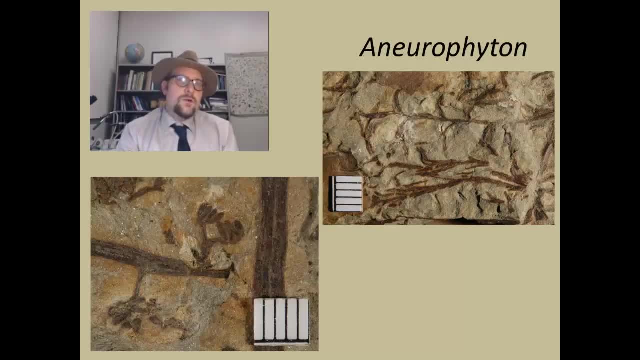 This is a Devonian plant. this is a Neurophyton. A Neurophyton is believed to be a tree like plant, and it grew and has split like sporangia. These little structures down here that you see in this fossil, these are the sporangia. 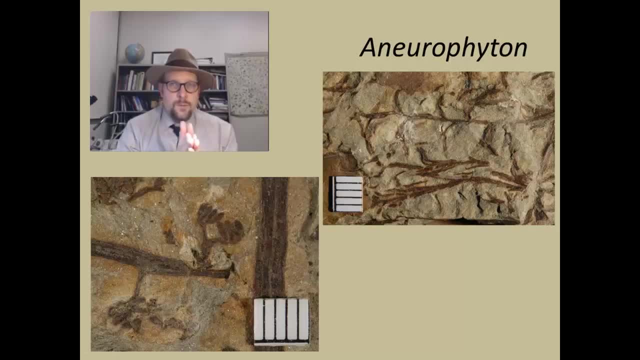 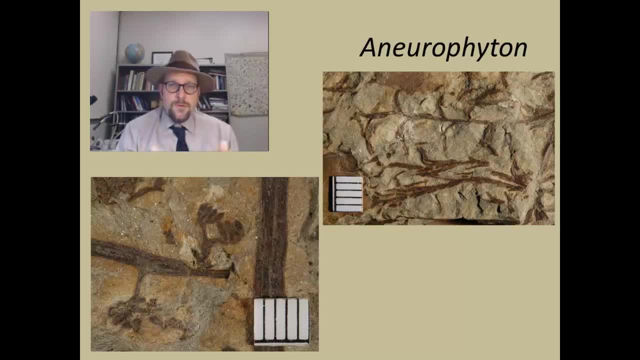 appear to be a male or a female sporangia. The spores are small, so we are not seeing a plant with a mega sporangia condition, like we saw in one of its early steps. What makes a Neurophyton really interesting is that it contains gymnosperm-like wood. 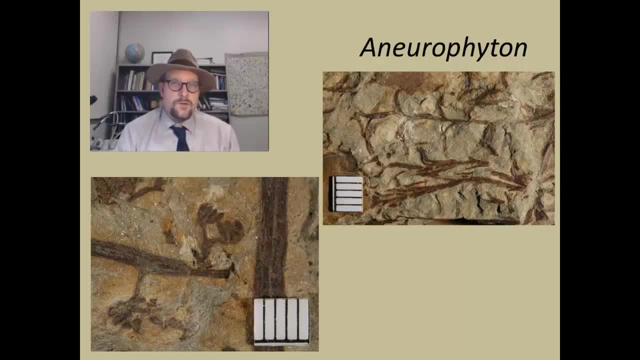 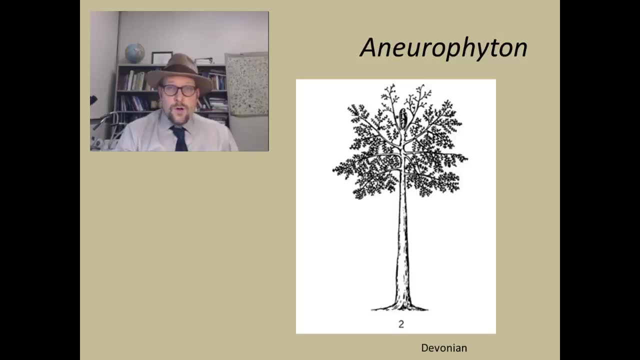 protosteel surrounded by secondary xylem- xylem composed of trichids and ray cells that come out. This is unique and allowed Aneurophyton to grow rather high like a tree during the Late Devonian, very early in the history of plants. 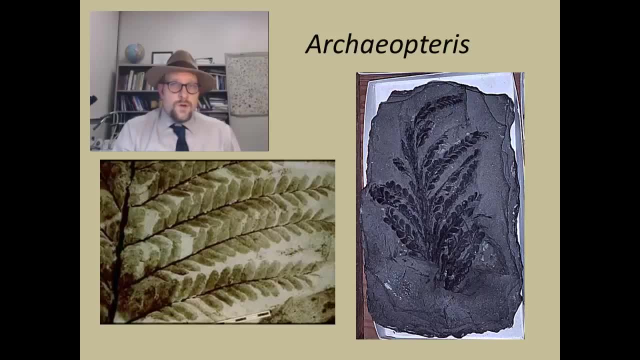 The next fossil is the tree-like Archaeopteryx, which was for many years recognized by fern-like leaves and often regarded as an early fern. The leaves are very similar to modern ferns, with each leaf extending from a branch. Many early paleobotanists regarded these as early ferns from the Late Devonian and were 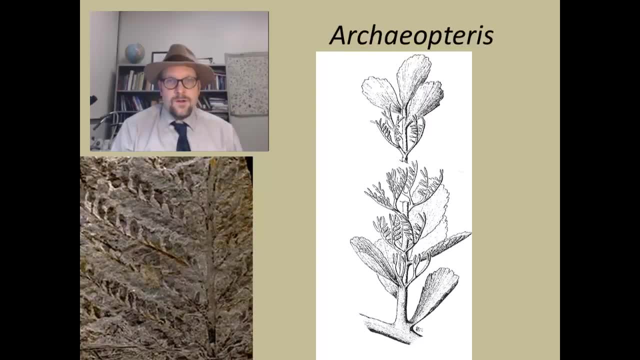 remarkably common fossils Like ferns. Archaeopteryx produced free spores from the sporangia along the leaves. These are these little structures. Here you can see the sporangia that produce spores. You can divide the leaves into fertile leaves. these are the leaves with the spores and 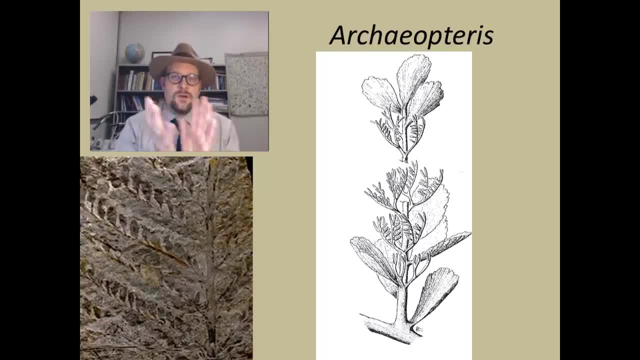 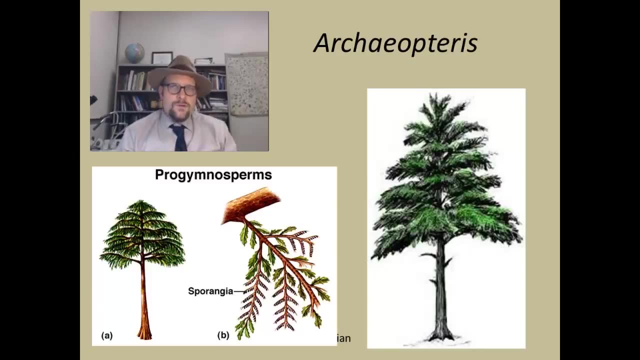 the infertile leaves are the leaves without the spores. They are arranged in an interesting spiral pattern on these leaves. A major discovery was made when the oldest fossil wood placed in the wood-formed taxa called Kalazalon was discovered in association with the leaf-formed taxa. 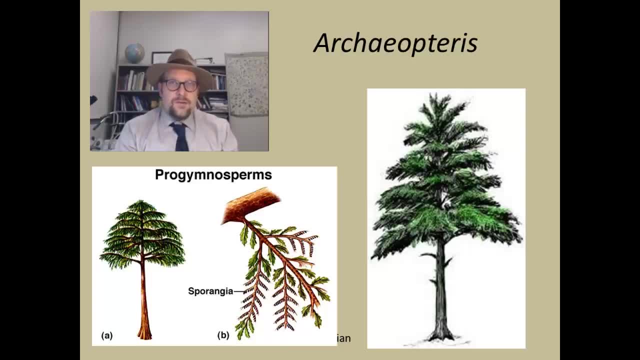 Archaeopteryx. hence Archaeopteryx had gymnosperm-like wood, much like a Neurophyton. This was a pretty radical idea that here we had this fern-like plant with fern-like leaves that also had gymnosperm-like, wood-like xylem in the trunks of these trees. 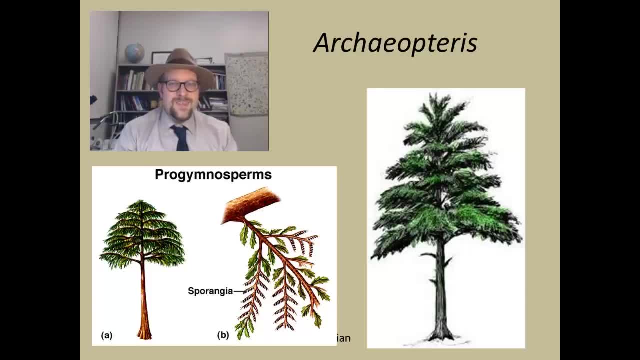 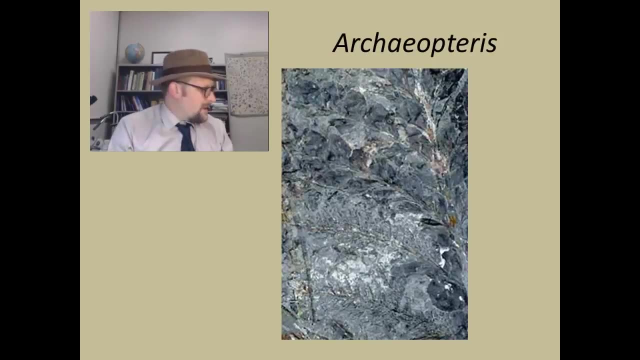 This tree is pretty interesting because we are still in the Late Devonian, so this is one of the earliest trees we are starting to see on the planet. Here is another fossil of Archaeopteryx and, wow, what is this thing right down here? 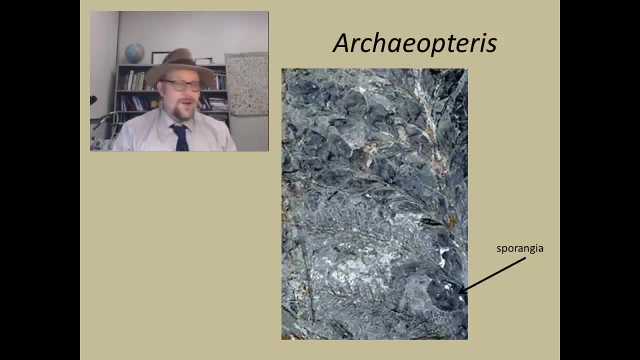 It's a different looking sporangia on a fossil branch. Some forms of Archaeopteryx have two types of sporangia, Hence they are Hedrospori. that means they have female and male sporangia on the plant. 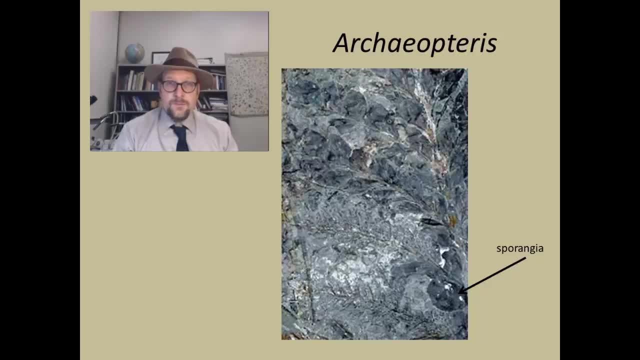 These are Megaspores and these are larger female sporangia. So far, scientists have found there are two species of Archaeopteryx with different sex sporangia, just like what we predicted, and we are still way back in the Devonian 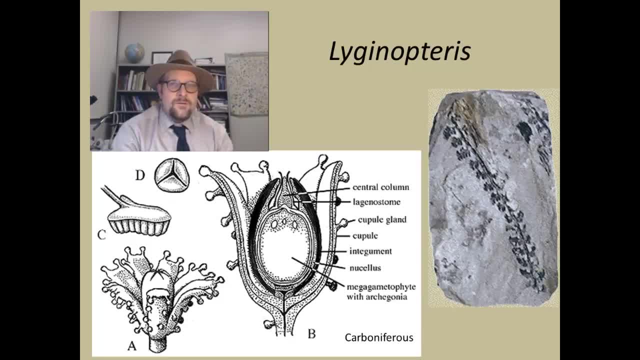 Alright. Next Let's get into the Carboniferous with a fossil called Lingenopteris, which is commonly found in cobalt. This is a vine-like plant and it has bifurcating leaves. The plant has microsporangia that produce trilent prepollen. 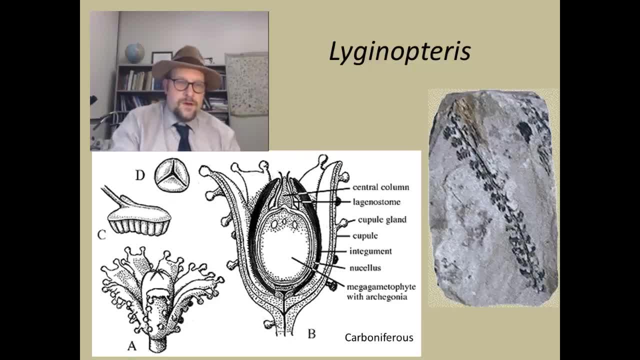 Trilent means that the pollen is of a tetrahed of cells. as you can see in this figure labeled D from the textbook, The plant also has an ovule, So here is the ovule. this is pretty cool. So here we have. this is the gamiphyte, the female gamiphyte, which here they have labeled. 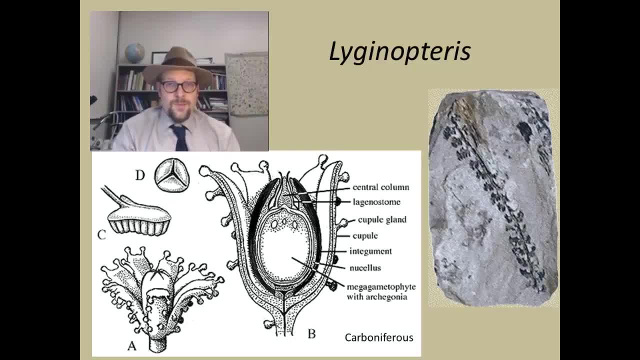 as the megagamiphyte, with the archegodium there, And so that is going to have the cell that is going to represent the egg cell And it is in this really interesting cupula, So it is retaining this structure on the plant. so the gamiphyte is on the plant and it is. 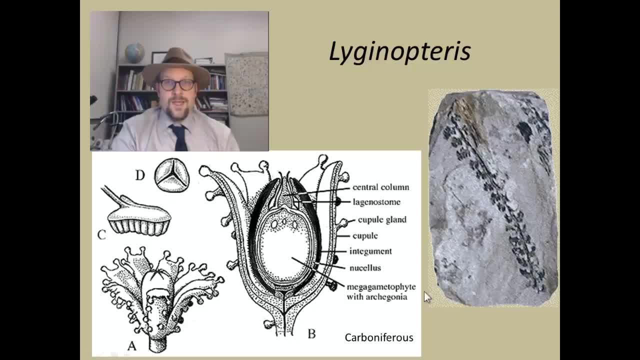 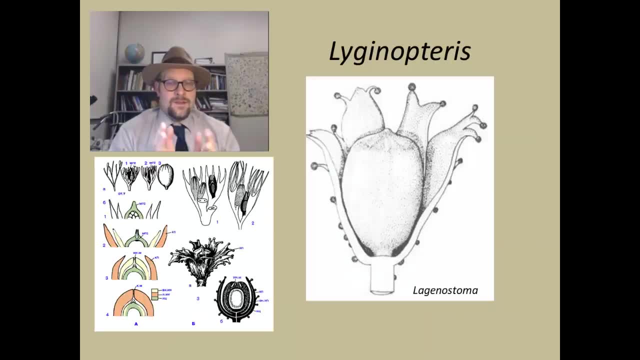 opened up And we have this narrow column on the top that is going to catch those little pollen grains when they are released from the plant. Now what is really interesting is that these ovules, when they are fertilized, will produce real seeds. 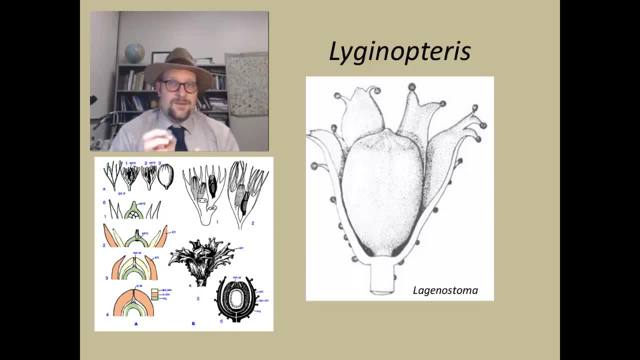 So here is a picture of one of the earliest seeds we have. This is the form taxa, the seed form taxa for Lingenopteris, which is called Liginostoma, And this is the seed name for the structures found in these plants. 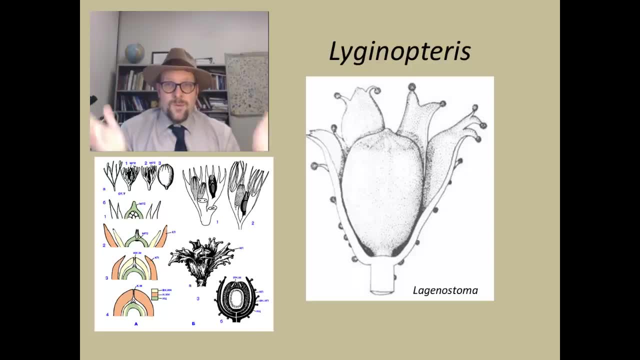 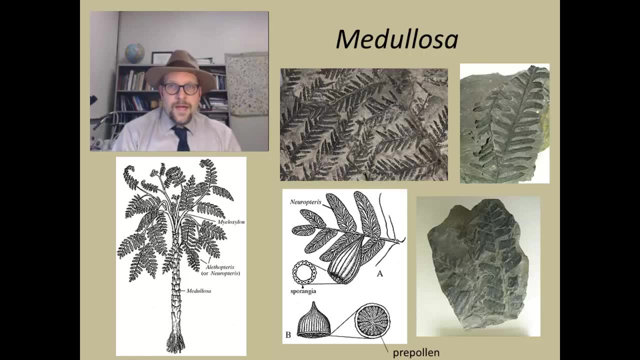 But this is what the first seeds look like. We have seeds Now. the next fossil plant we are going to look at is Meldolosa, which is a plant from the Mississippian or Luracarboniferous. It has an interesting woody structure.